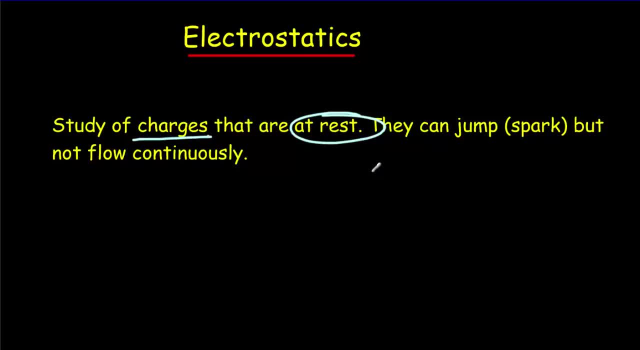 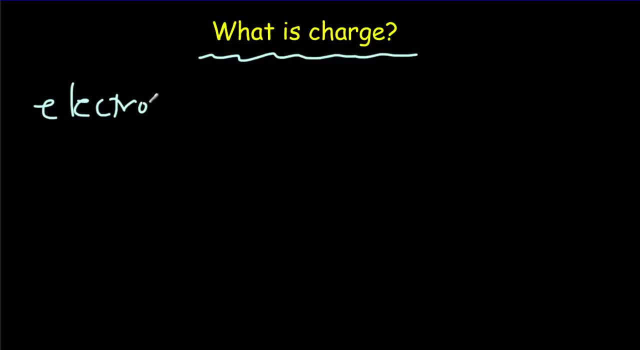 so when we're studying electricity, we're really studying the currents. What exactly is charge? Well, we know it's coming from the electrons and the protons, And the electrons have a negative charge. the protons have a positive charge. What we're generally referring to when we talk about charge is a deficit or a surplus. 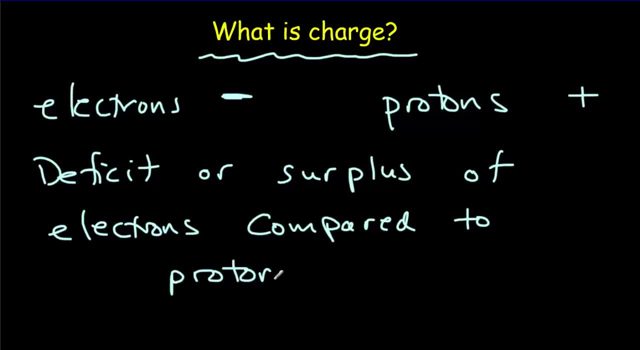 of electrons compared to protons. So if we have two protons and two electrons- positive and negative- cancel each other out and we have no charge. But if we've got three protons and two electrons, we're going to have a small positive charge. 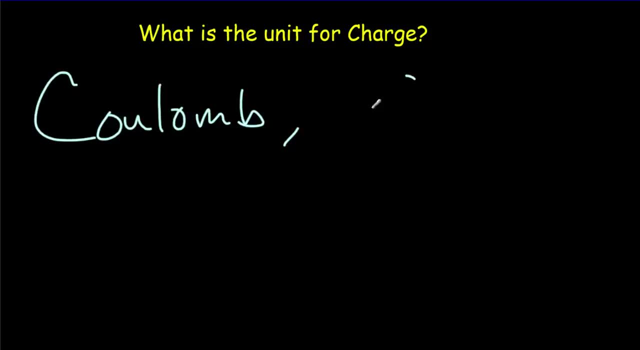 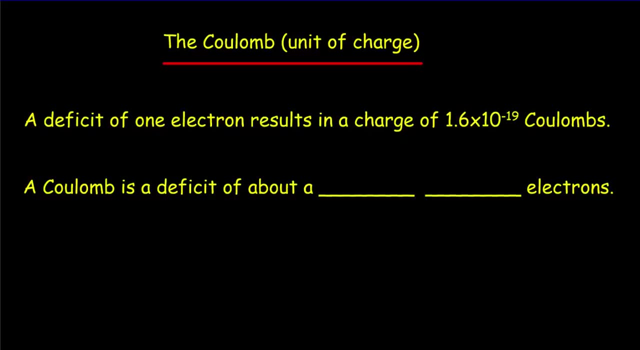 The unit for the charge is called the coulomb, and we give it the letter C as a symbol. Now, what exactly is a coulomb? It turns out a coulomb is a very big charge If we have a deficit of exactly one electron, that is, we have one more proton than electron. 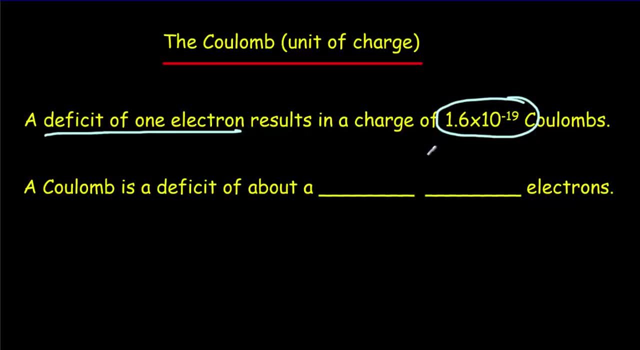 then we get a charge of only 1.3.. That's 6 times 10 to the minus 19 coulombs And that means that a full coulomb would be 1 over that very small number of excess electrons. That's going to be about a billion billion excess electrons in order to make a coulomb. 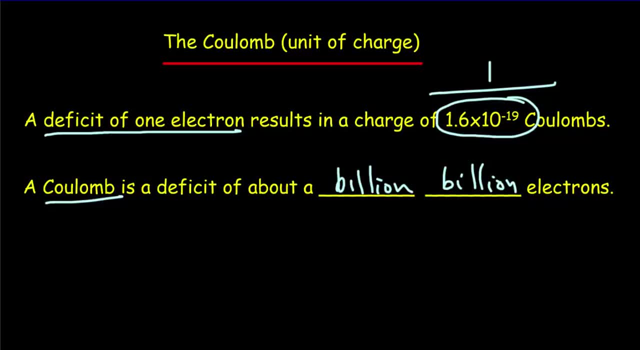 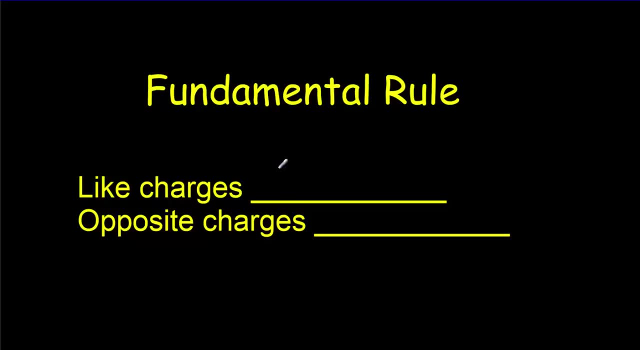 So a coulomb in fact is a large amount of charge. We have a fundamental rule of electrostatics and that is that like charges, it will repel, Whereas opposite charges attract. So if you've got two electrons, they're going to push each other away. 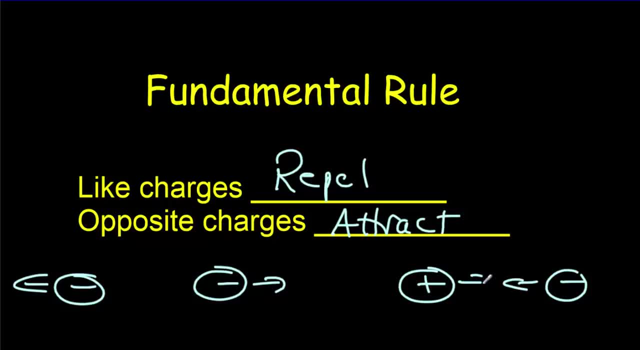 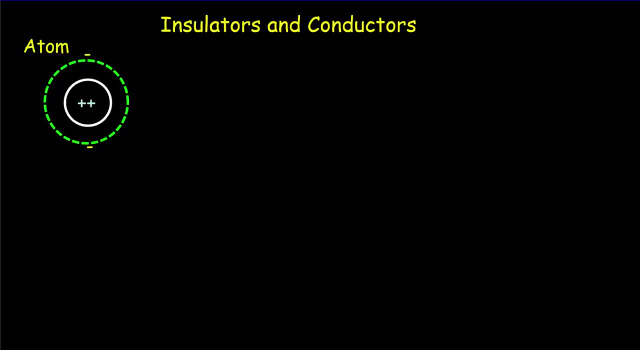 But if we've got a proton and an electron they're going to attract each other. The idea of charge leads into a very important idea in electricity and that is the difference between insulators and conductors. So in an insulator charge has a hard time flowing. 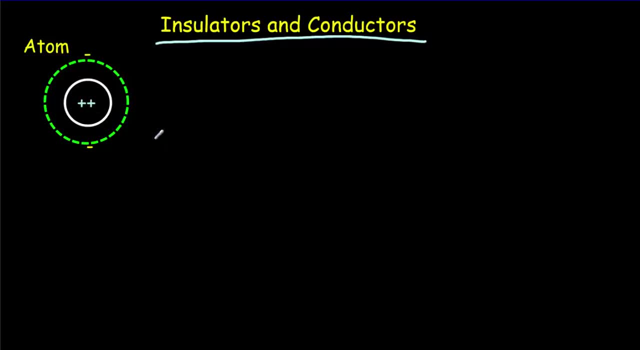 In a conductor, the charge flows very well, At least for our purposes. what that's going to mean is, if we've got an insulator, the electrons are going to be attached to the positive nucleus. It's going to be a strong bond there and your atom there is going to be balanced an.